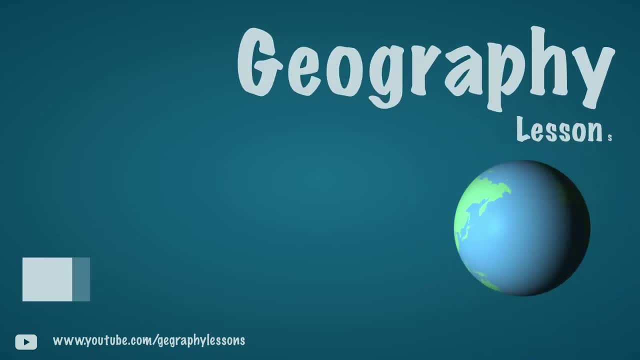 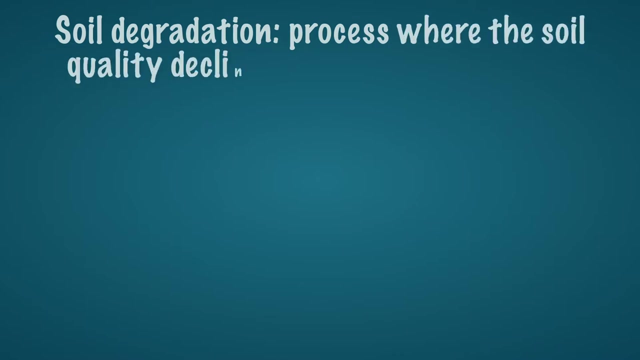 In this video, the causes and consequences of soil degradation are explained. The word soil degradation contains the word degrade. This is used when a decline in performance is explained. so it has gotten worse. This also applies to soil degradation. If the soil degrades, it is actually less useful, reducing the yields of food, timber or fresh water. 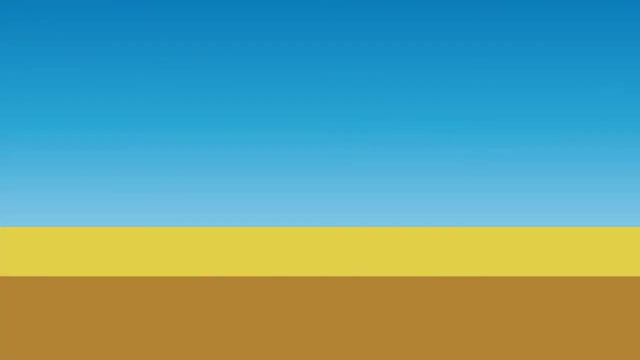 This may be because people have poorly maintained the land. Suppose crops grow in an area, People remove the vegetation, like trees and plants, For example. people need the wood. there is deforestation. People can also graze cattle and the cattle eat all the vegetation. this is called over grazing: Vegetation disappears. 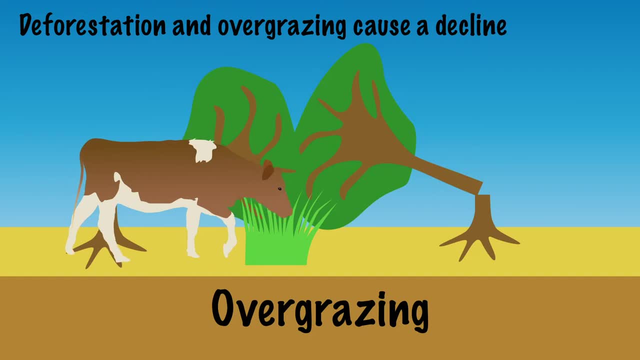 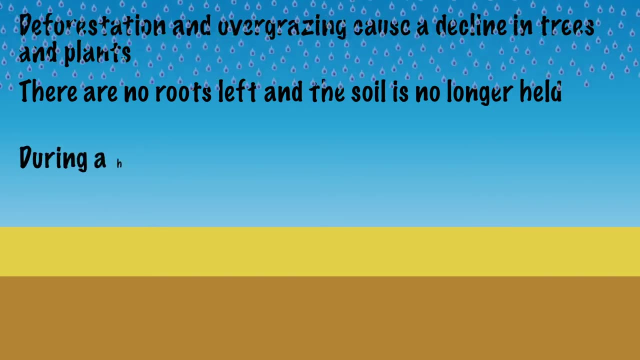 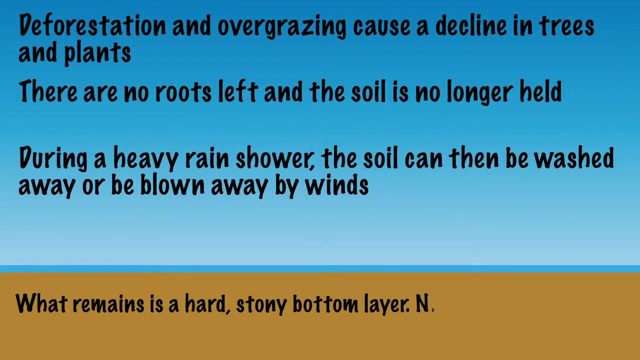 in the event of deforestation or over grazing. Normally, roots Hold the soil, but because there are no roots left, the soil is no longer held. During a heavy rain shower, the soil can then be washed out away. This is called soil erosion. What remains is a hard, stony bottom layer. New plants can't. 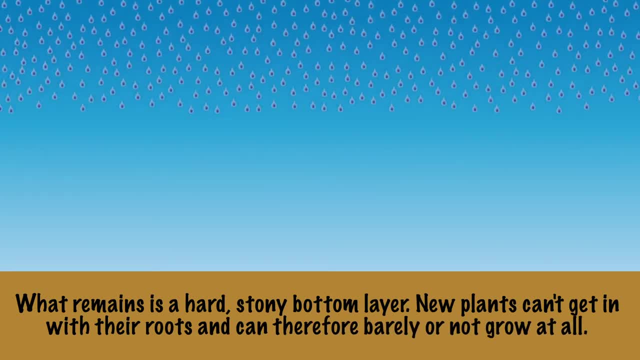 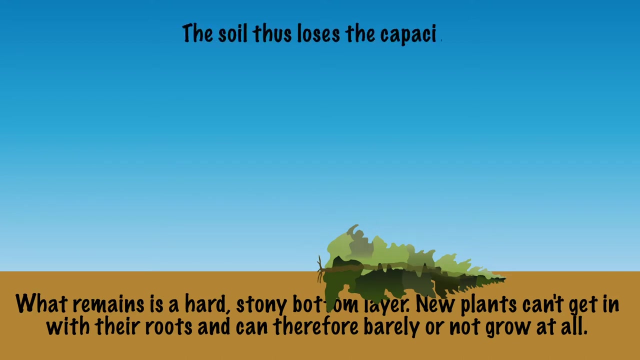 get in with their roots and can therefore barely or not grow at all. Also, with a new rain shower, the water cannot enter the soil so that it washes over the surface. Because there is no water available in the soil, vegetation can grow even more difficult. The soil thus loses the capacity. 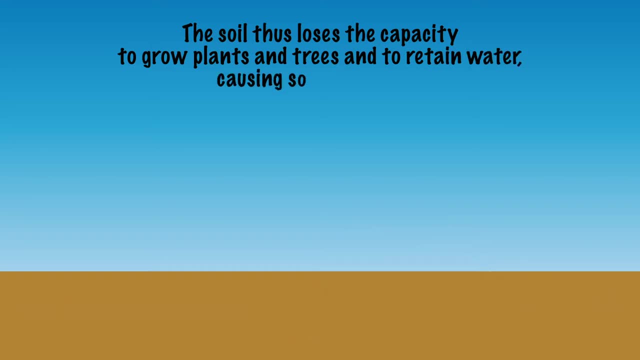 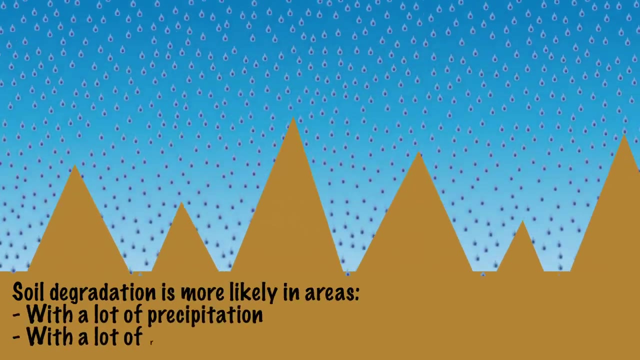 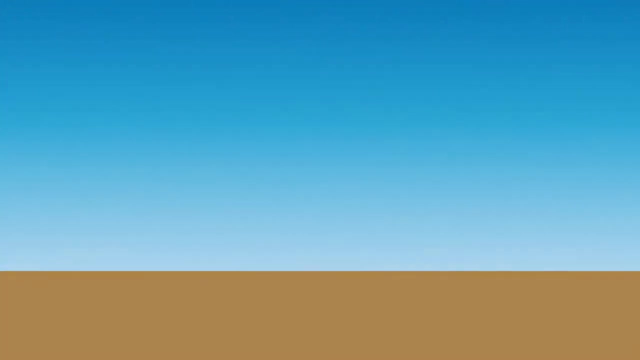 to grow plants and trees and to retain water, causing soil degradation. In areas with a lot of precipitation and a lot of relief, the soil can wash away much more easily. More water is available and because the bottom is steep, it will wash away more easily. Another form of soil: 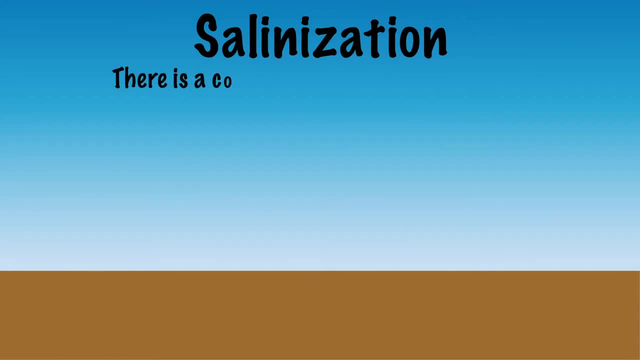 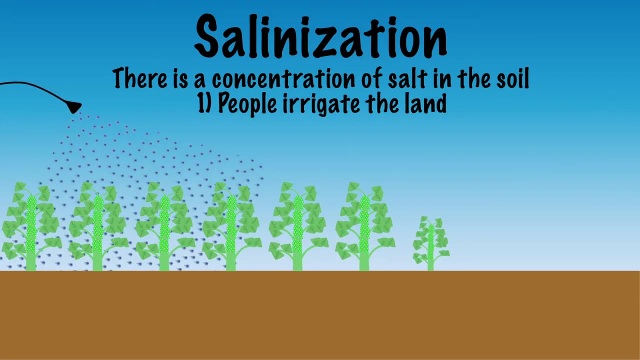 degradation is salinization. This means that there is a concentration of salt in the soil. That's because people irrigate the land. They use a lot of water in warm and dry areas on agricultural land. This is a big problem. A lot of people have a lot of water in warm and dry areas on agricultural land. 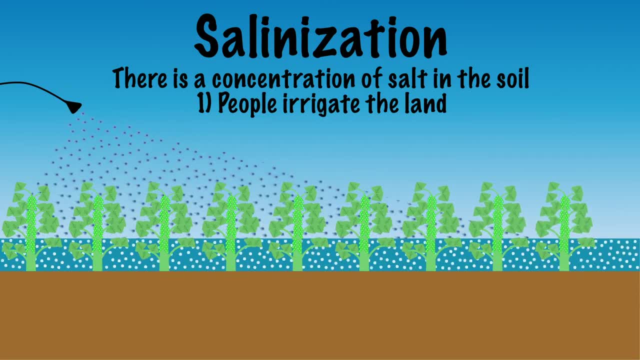 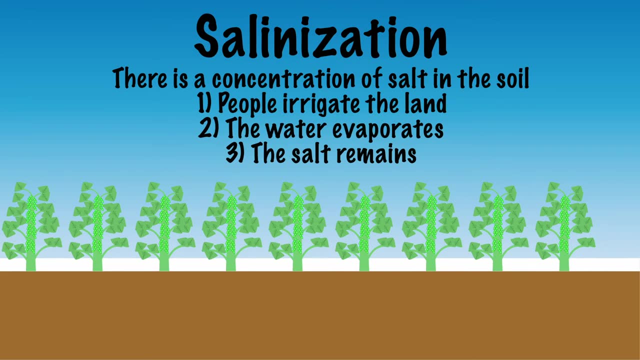 lands, But even drinking water contains a little bit of salt. If the water evaporates on land due to the heat, the salt remains because it does not evaporate. The cause of salinization isn't because the water washes away, but because it evaporates In this way. 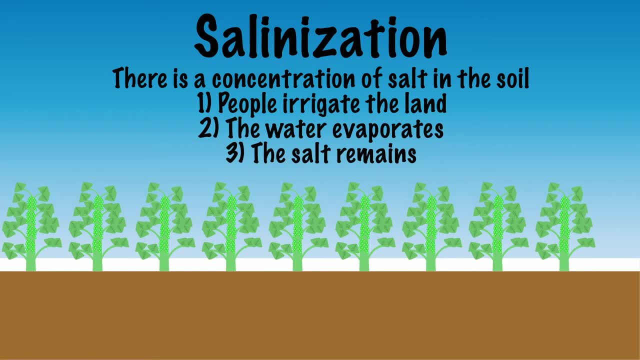 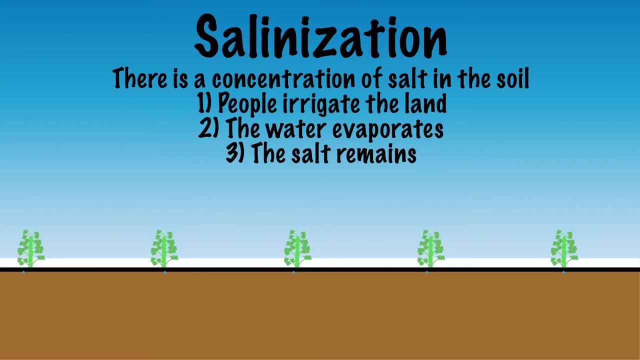 salt accumulates, decreasing plant growth. As a result, the yield of agriculture is decreasing and thus there is soil degradation. One solution may be to improve the efficiency of irrigation channels, so that less water is needed and therefore less salt ends up on the land.